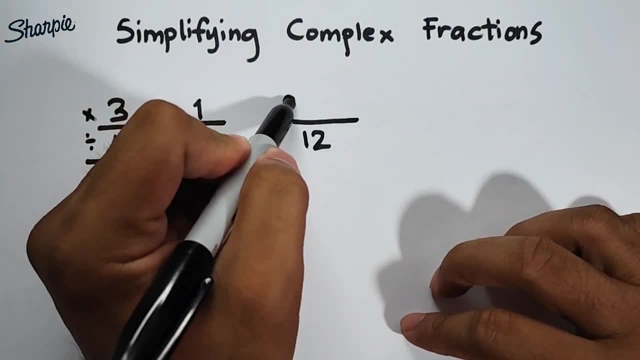 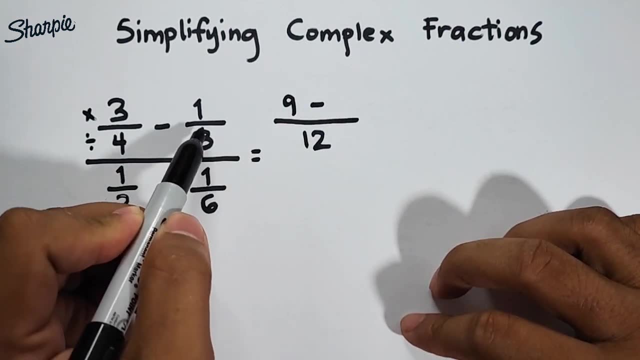 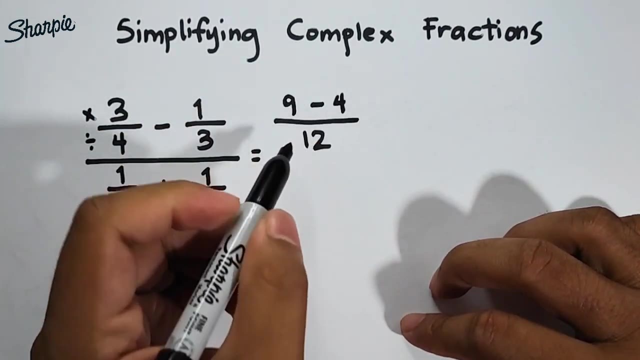 And then times 3,, that is equal to 9.. Minus 12, divided by 3,, that is equal to 4.. Times 1,, that is equal to 4.. So on Tunte, we're simplifying the numerator. 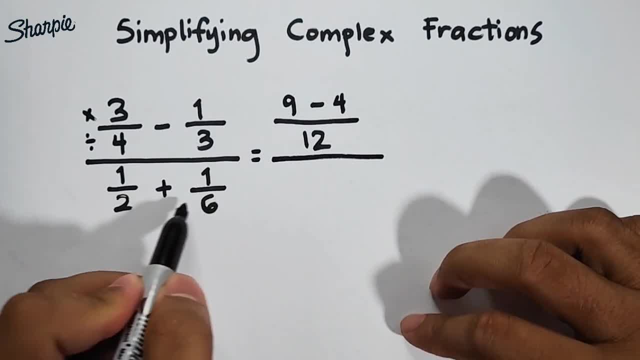 So next is your denominator: 1 half plus 1 over 6.. So what we need to do is to get the LCD of 2 and 6, which is 6.. And then 6 divided by 2 is 3.. 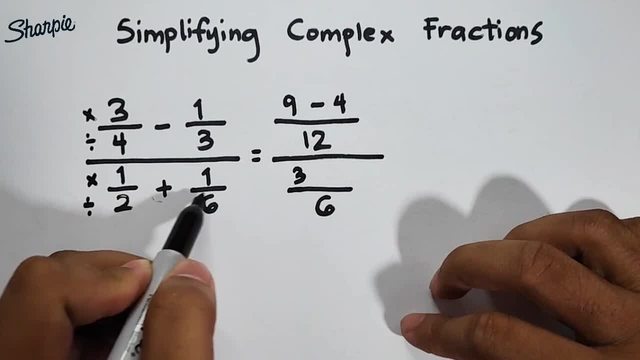 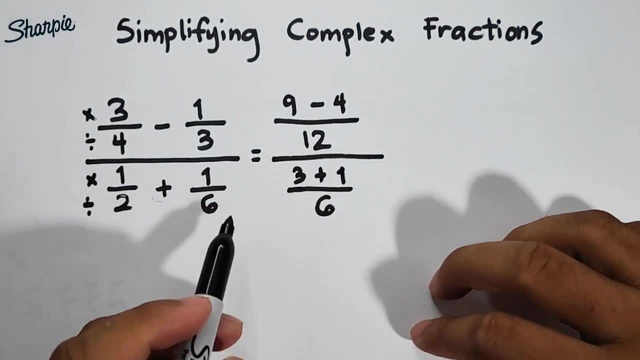 Times 1, that is 3.. Then copy this operation: plus 6 divided by 6 is equal to 1.. Times 1, that is same, Simply 1.. So all we need to do for this part is to simplify the numerators. 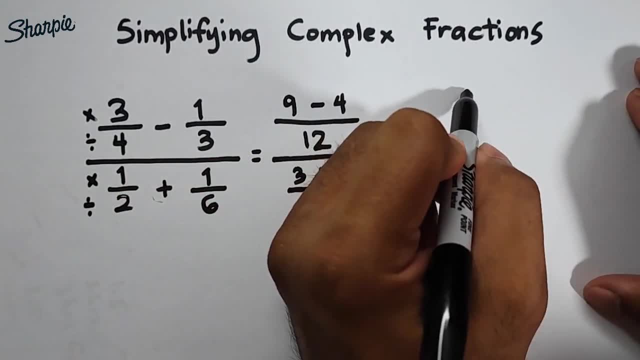 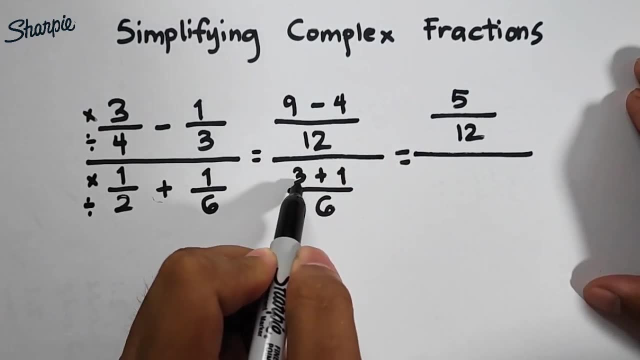 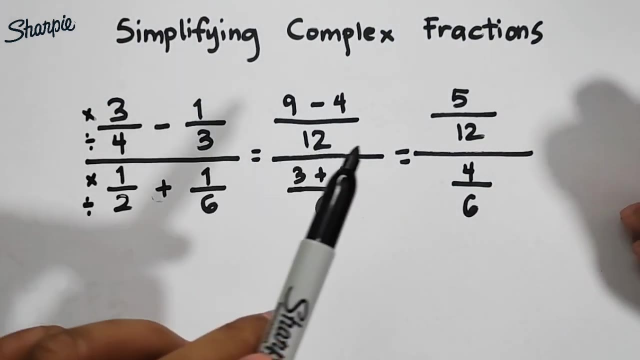 9 minus 4 is equal to 5 over 12.. And then originally all over 3 plus 1, which is 4 over 6.. So what we have now is this: given fraction, We have 5 over 12, from 3 over 5.. 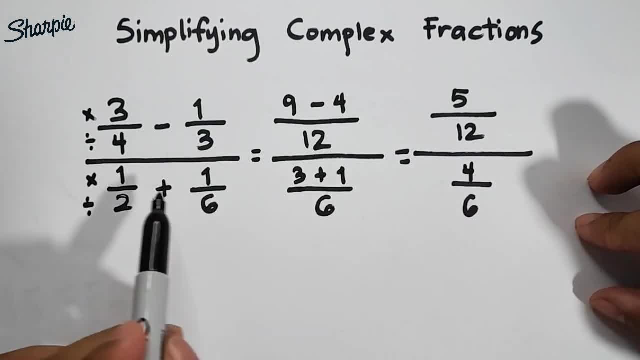 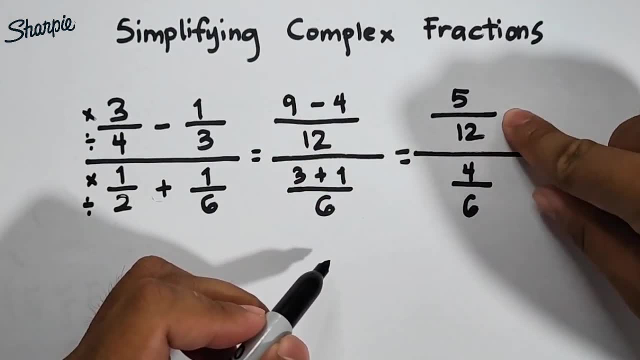 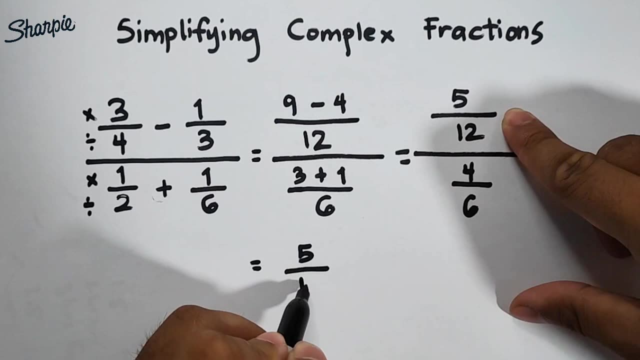 4 minus 1 over 3, all over 4 over 6, from 1 half plus 1 over 6.. So what we need to do here, as you can see this one is division. So we will copy: 5 over 12 over 4 over 6.. 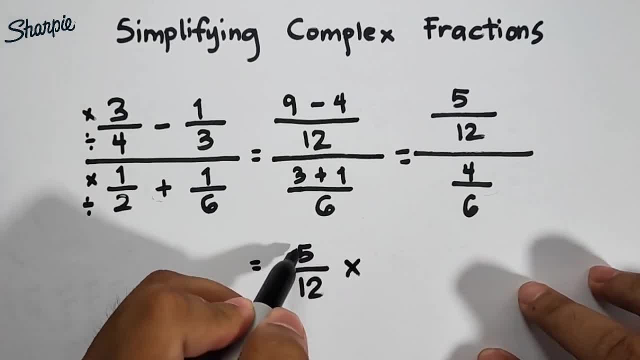 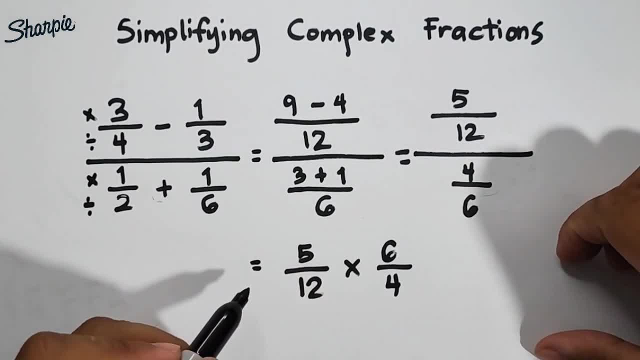 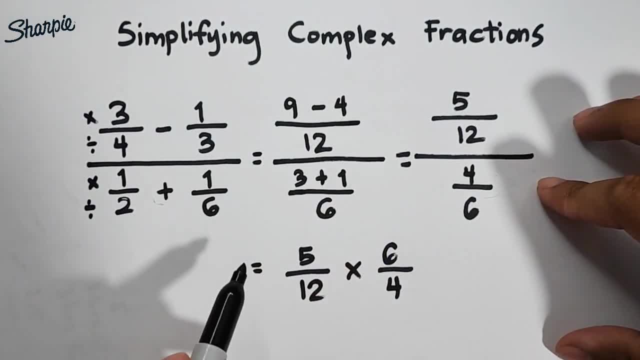 Now, instead of doing that, we can use cancellation. As you can see, we have here 12 and 6, wherein their greatest common factor is 6.. So we can eliminate this 6 and it will become 1, because 6 divided by 6 is 1.. 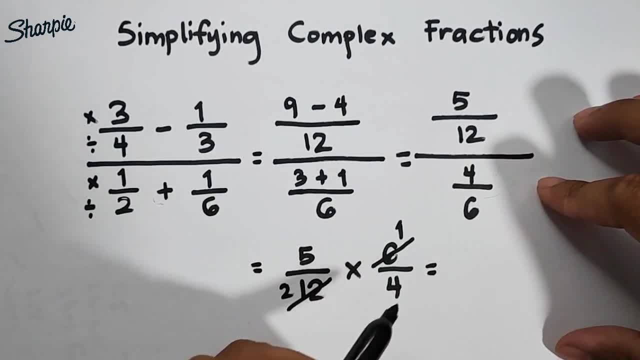 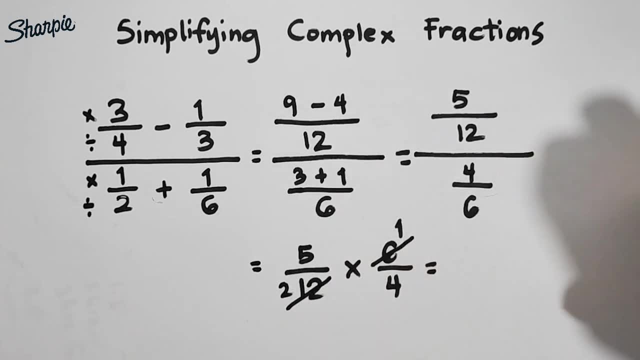 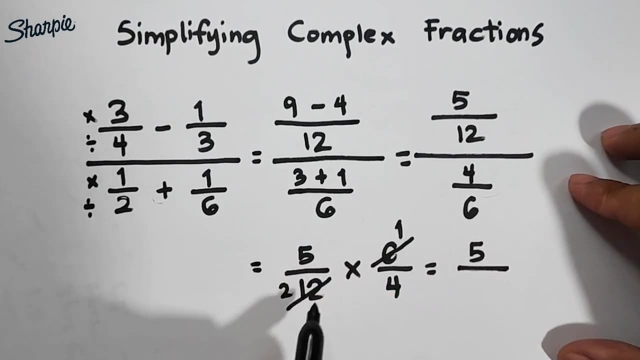 And then 12 divided by 6 is 2.. So the purpose of it is to simplify or to lessen the number that we're going to use in this kind of formula. So what we have now in the numerators is 5 times 1, which is equal to 5, over 2 times 4,. 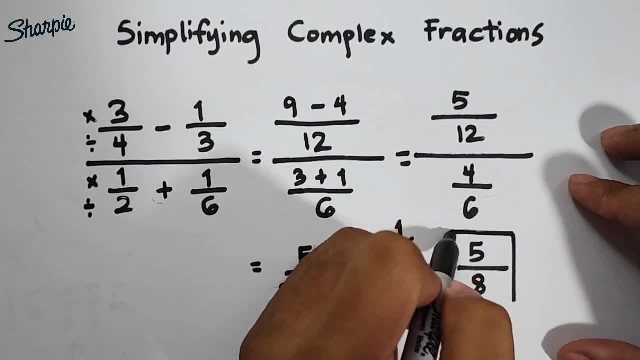 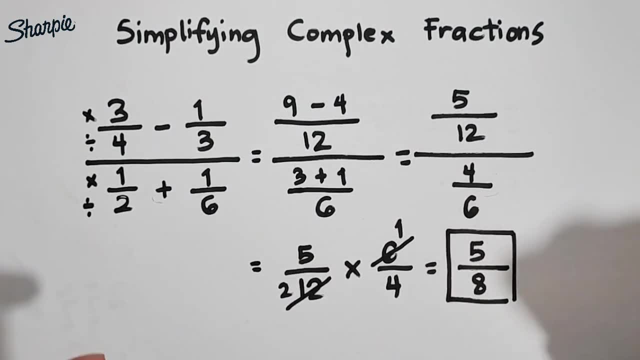 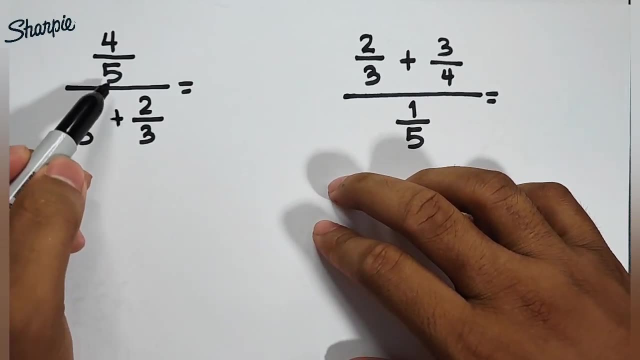 which is equal to 8.. So this is now the answer for item number 1.. In the next part of our video, I will give you another example wherein we will simplify complex fractions. Now let us continue with this second example. We have 4 over 5, all over 1 over 5, plus 2 thirds. 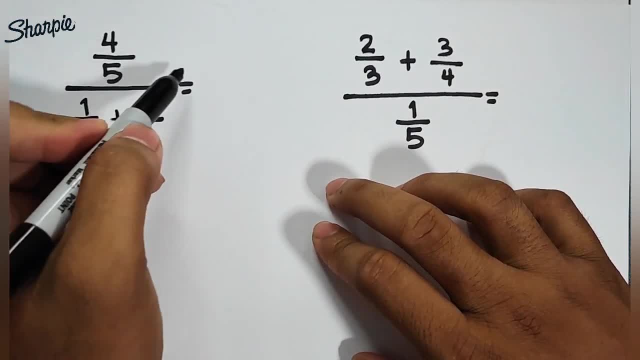 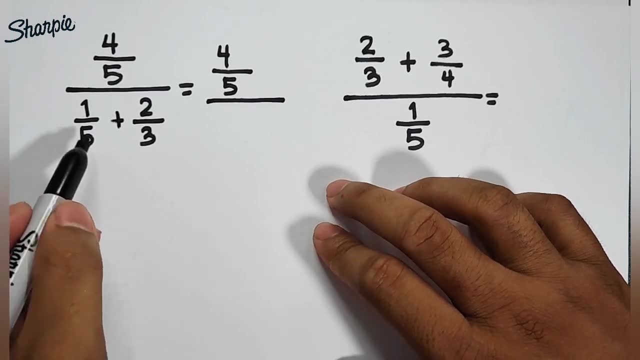 So, as you can see in the numerator, we only have 4 over 5.. So we will copy that: So 4 over 5.. What we need to do is to simplify this denominator. So the denominators are 5 and 3.. 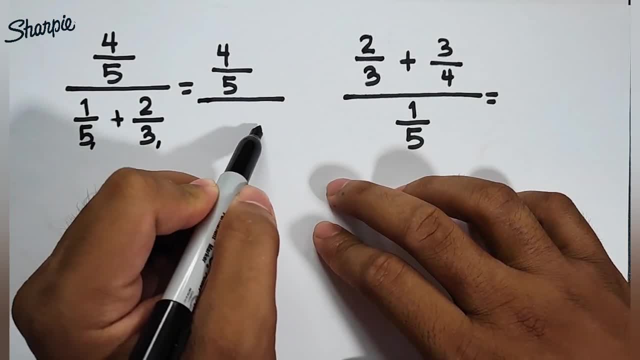 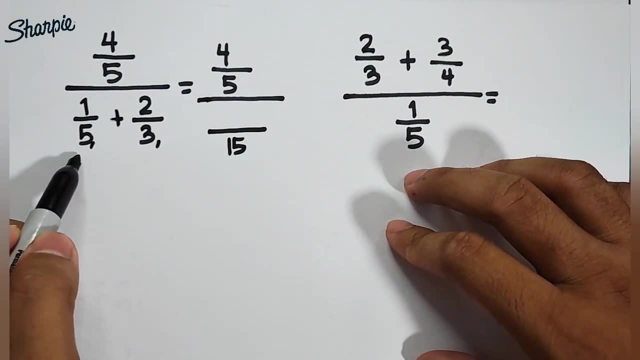 So what will happen is that the LCD is 15.. So we have to put 15 here, And then let's do the common way. 15 divided by 5 is 3.. Okay, Times 1,, that is equal to 3.. 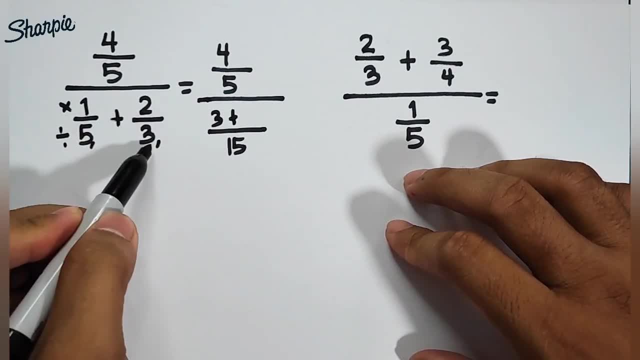 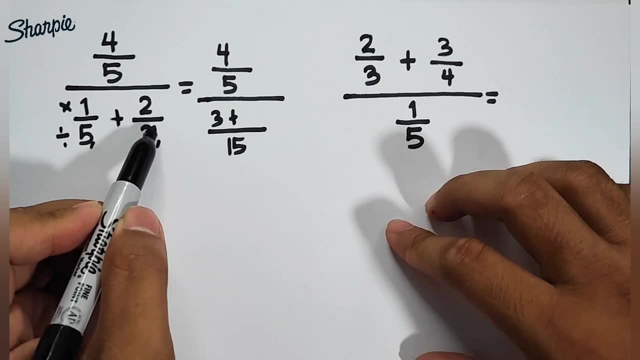 Then copy addition For the next fraction, we have 15 divided by 3, that is equal to 5, times 2. That would give us the answer of 10.. So we need to simplify this And it will become: 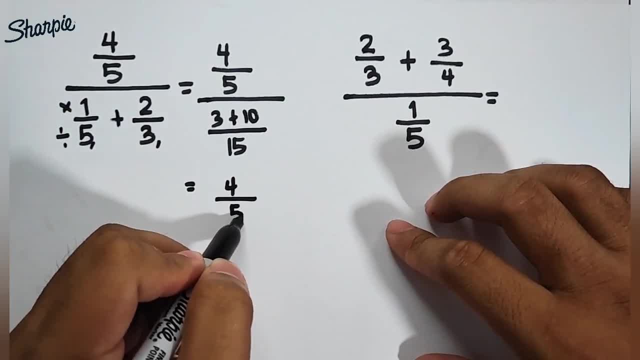 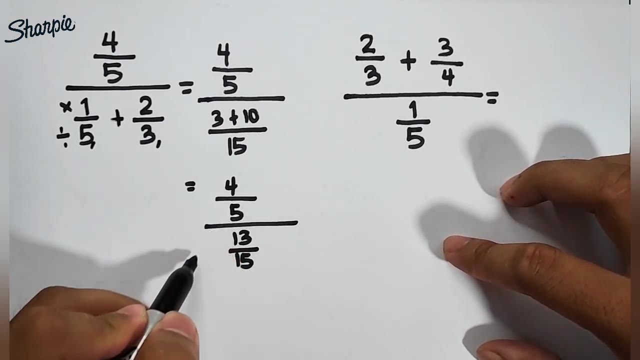 Copy 4 over 5.. You have 4 over 5, all over 3 plus 10,, that is, 13, over 15.. So what's next after this is that we will get this 4 over 5.. Copy them. 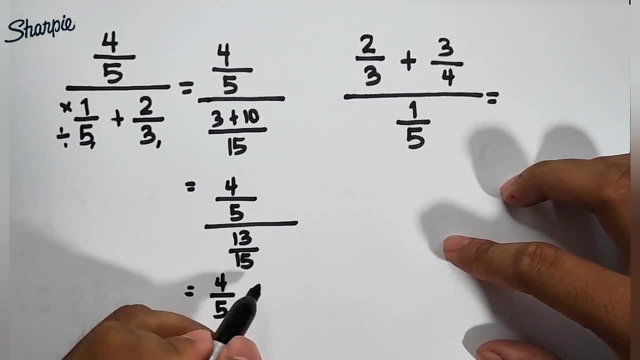 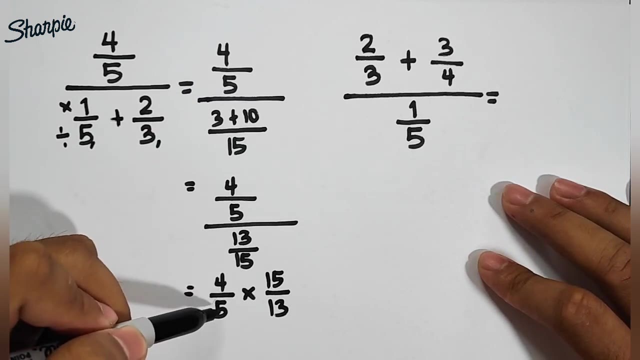 Copy the fraction 4 over 5. And then multiply by the reciprocal of 13 over 15,, which is 15 over 13.. So you need to observe the given fraction. okay, As you can see, we can do the cancellation method by 5 and 15, because their GCF is 5..